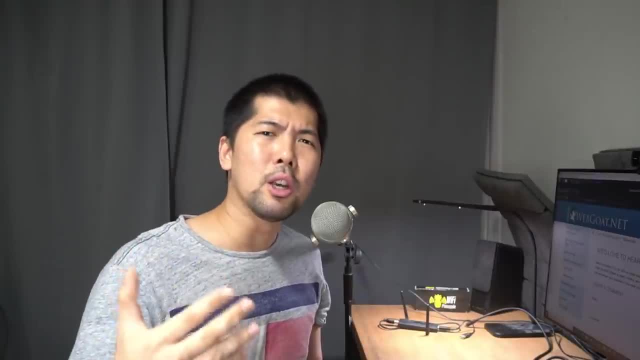 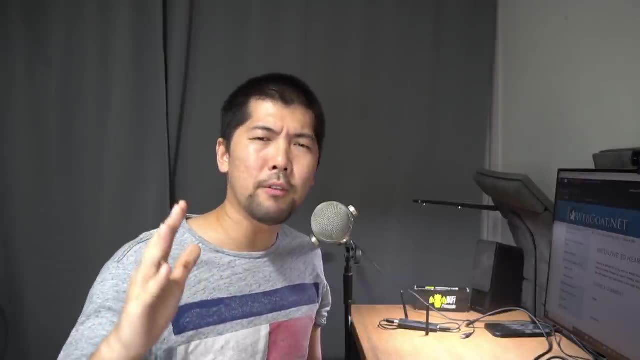 home lab environment. By the way, remember to subscribe to the channel so that you can learn all about ethical hacking and penetration testing And like the video, if all this content has been valuable and insightful for you, So, without further ado, let us get started on today's tutorial. 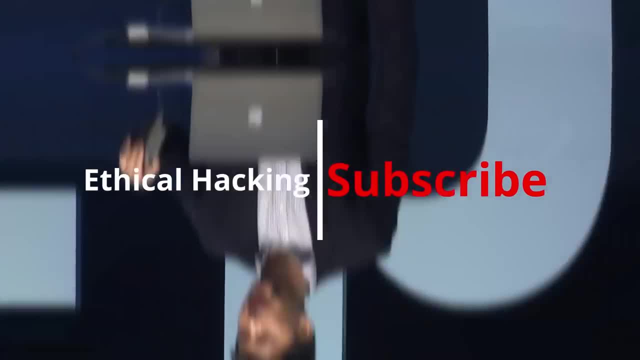 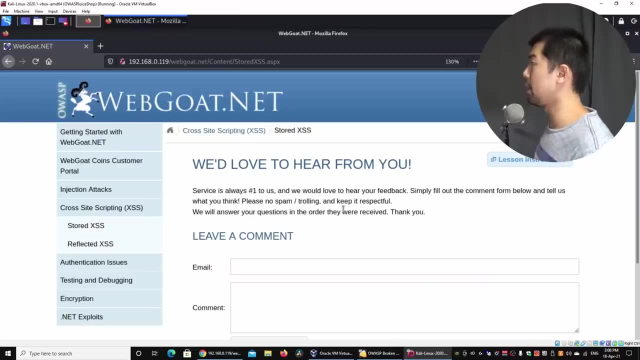 So right in front of us we have Webcodenet, which is a vulnerable web application system for us to perform our penetration testing and all the ethical hacking techniques on this particular platform. And right here on the left side I have cross-site scripting and I can go ahead and click. 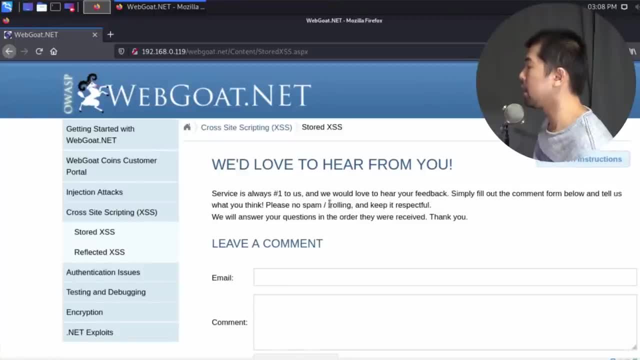 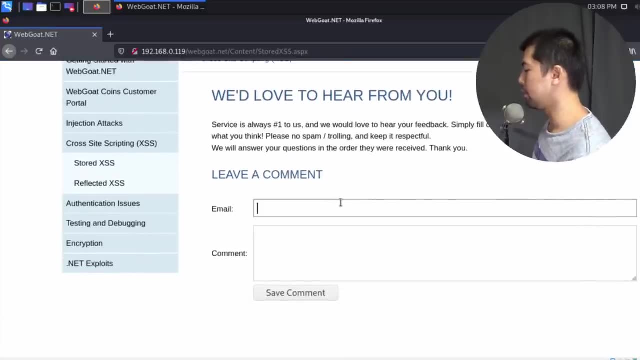 on the store XSS. So what does this do? right here is: it is very similar to any website. you go to right, Any sites where you can post a comment, post a review, And right here on the email, all I got to do now is go ahead and enter, say, my email, right: loyliangyang at loyliangyangcom. 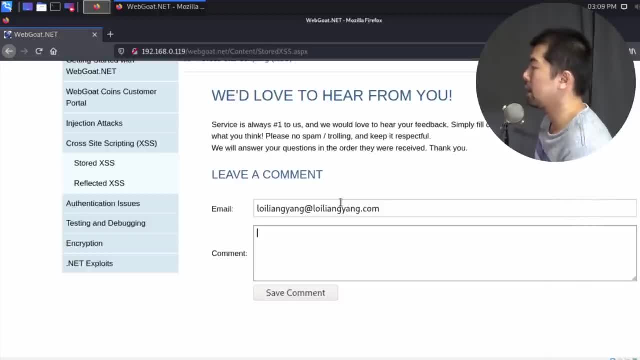 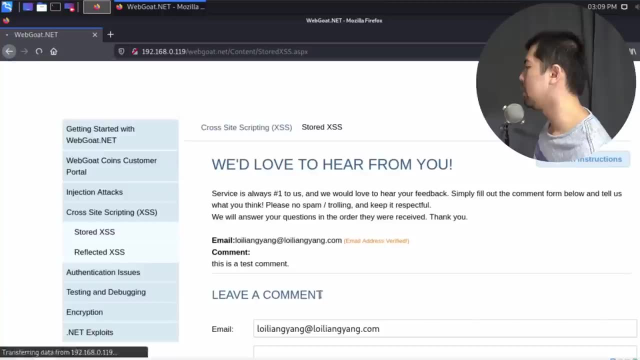 And all I got to do under the comment section is to go ahead and enter any comments. So, for example, I can enter: all right, this is a test comment. All right, go ahead and click save comment. So the first thing you want to do whenever you're encountering any features? 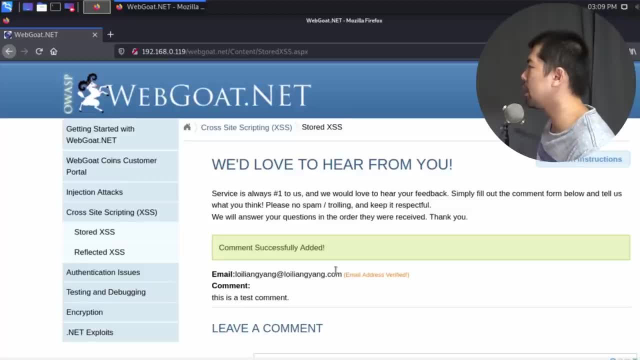 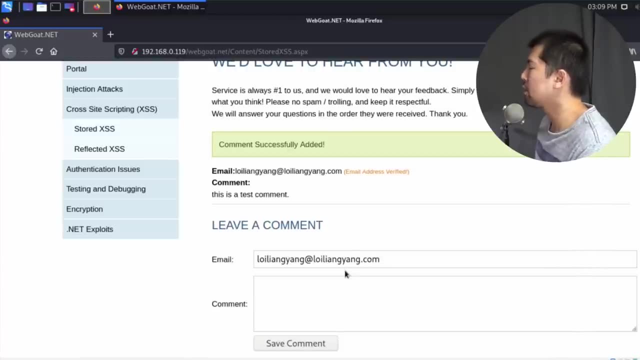 any functions is to go ahead and test it out and see what is considered as a normal behavior Next up. what you can do is now. this is the exciting part, This is the part where you are waiting for, And that is to test. 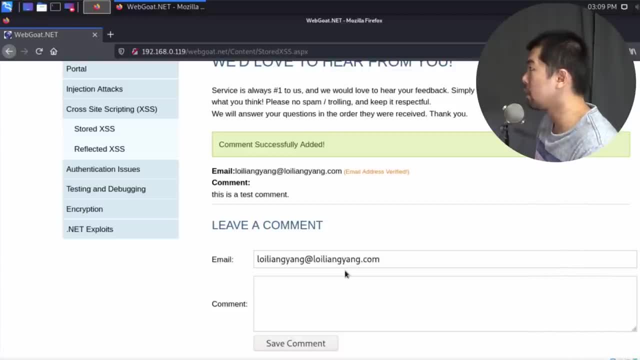 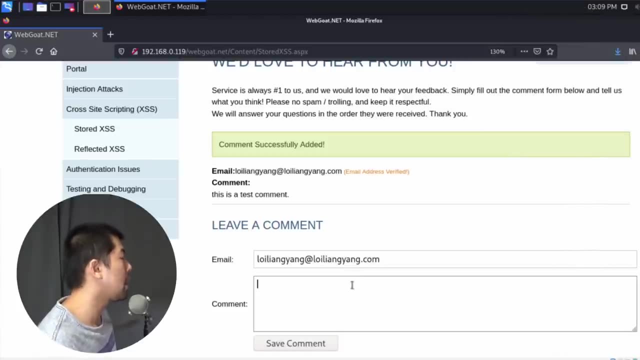 whether the comment or the email section is vulnerable to cross-site scripting, meaning are we able to plant our own script into the site. So what I can do now is to go ahead and enter under the comment section, or I can open script and I can close script And what I can. 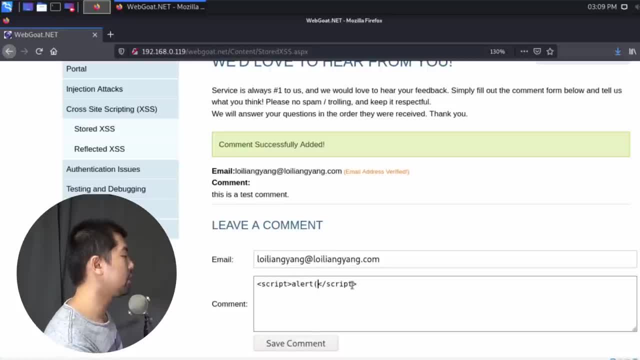 do right in the middle is to go ahead and enter an alert to see if this will get loaded as a script rather than as a website content. So I can go ahead and enter the following: hacked by LOI. All right, and I can close this with a semicolon. Go ahead and click save comment And. 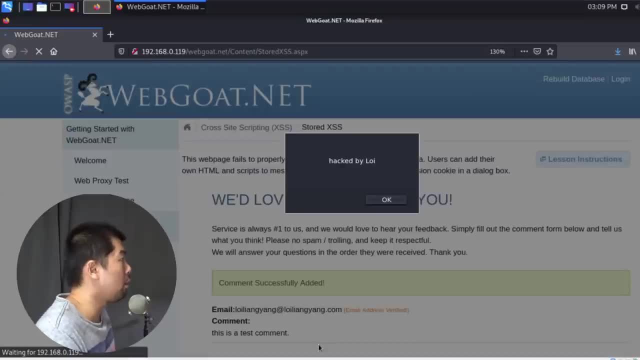 boom, we are in. Literally, our own code just got loaded just like that, As simple as that, And we managed to find one vulnerability in which we can now plant in our own malicious code. And it's pretty easy, isn't it? And that's scary, because you can literally try to find all these. 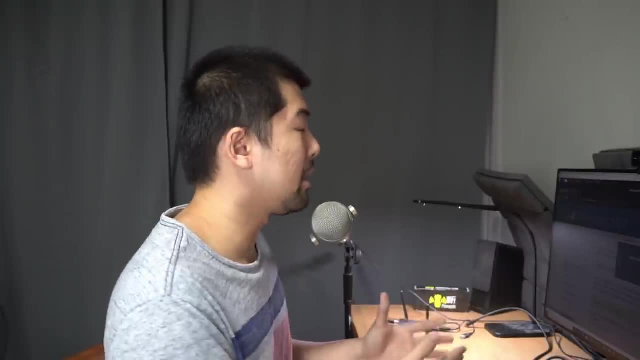 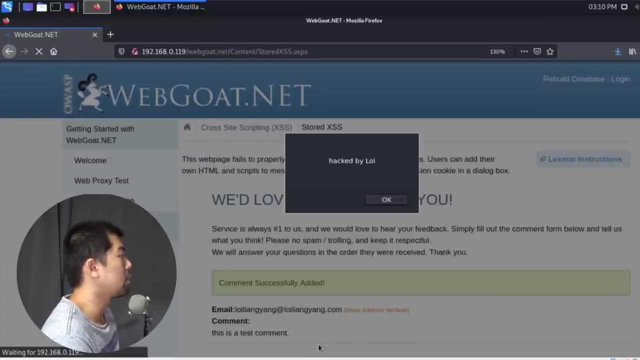 places text input box and you could try to plant any of this script in And that's it game over. We are in, So how can I demonstrate further about the ability for us to control the entire website? So go ahead and click OK on this And I'll go to the 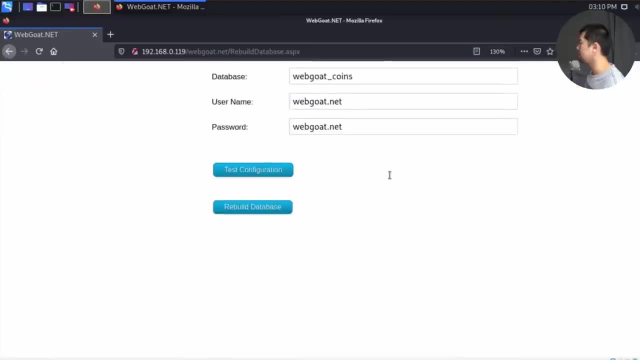 top left corner and I'll click under testing database. I'll scroll down further and I can click rebuild database. So the wonderful part about this on WebGoat is that whenever you screw up anything, all right, you can easily try to rebuild the entire database and you can start afresh. So 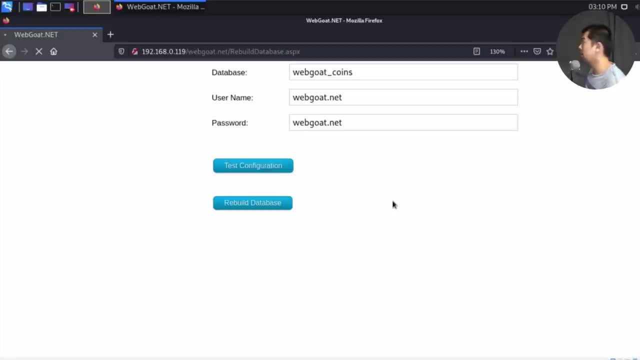 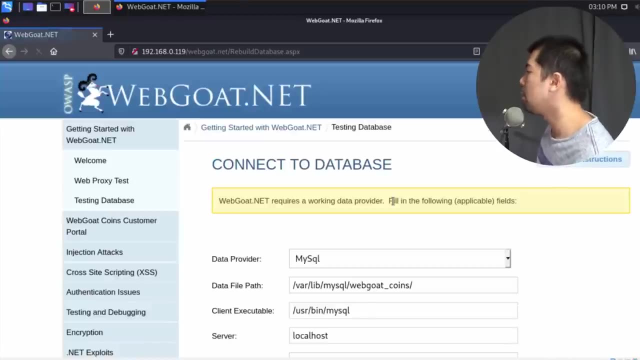 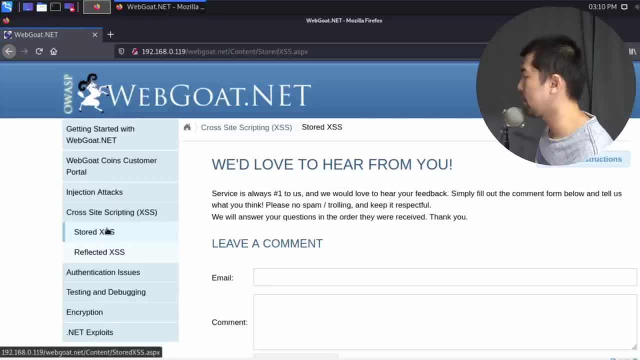 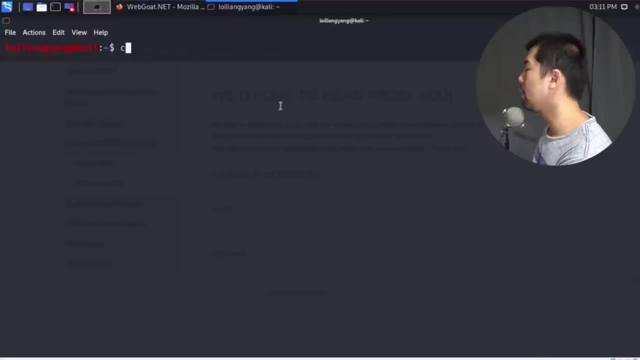 go back to cross-site scripting. Click under stored XSS And what I can do here now is to go ahead and open up browser exploitation framework. So I have already downloaded it and I can go ahead and see the BIF. all right, and I can enter LS to see all the files that are part of the BIF. 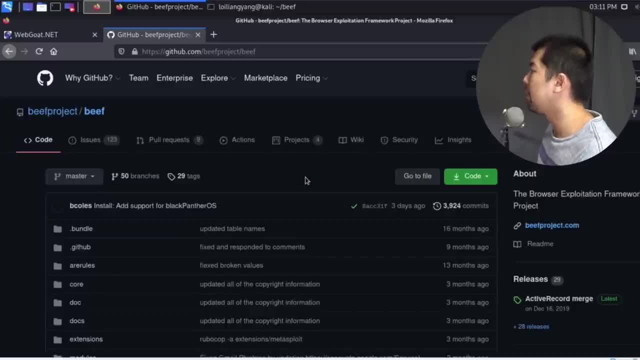 And you can easily do a Git clone on this, And this is the link to GitHub where you can download browser exploitation framework for you to run and implant all this malicious code and script into any website. So I have already downloaded it and all I got to do now 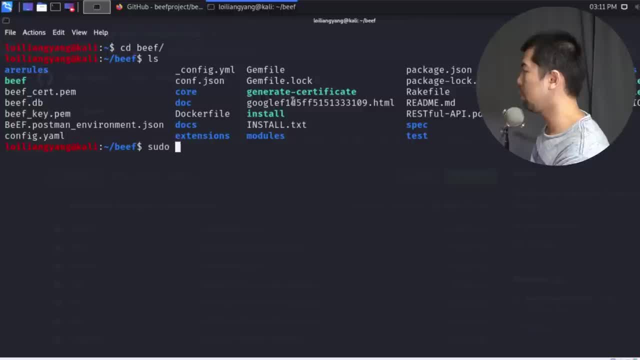 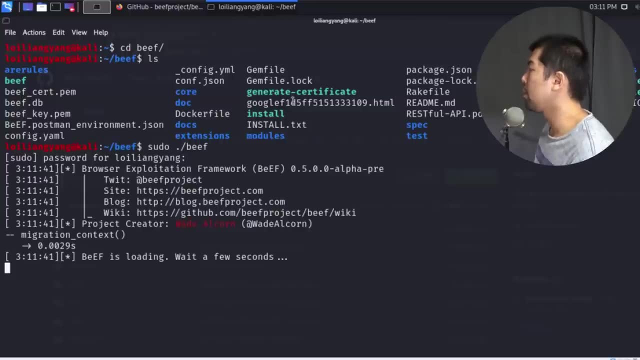 is go ahead and start up browser exploitation framework. So I can enter: sudo dot slash BIF. hit enter on this. enter your password for super user. hit enter and now we are loading up browser exploitation framework. So next up, what we can do here. the important part is this particular. 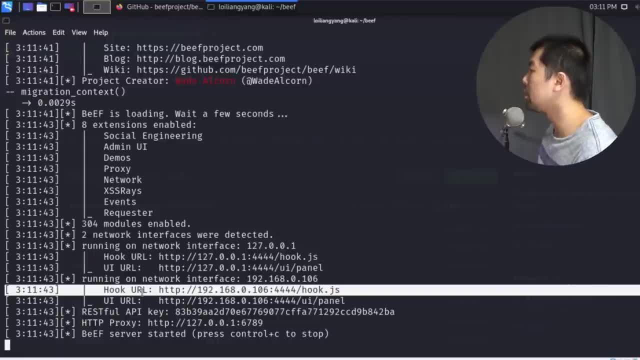 item, this particular row, which is called hook URL. So this is the JavaScript which will then allow us the ability to plan it into literally any website that you have found a vulnerability for cross-site scripting on. So all I got to do now is do a right click. 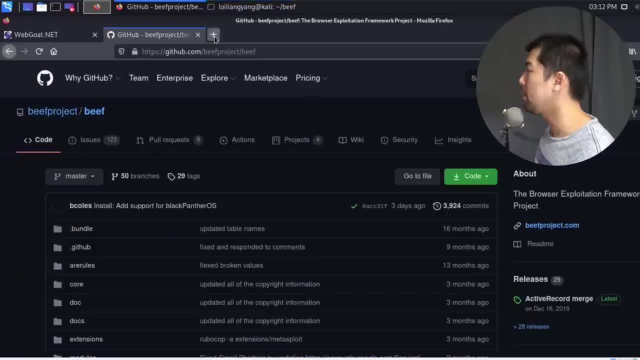 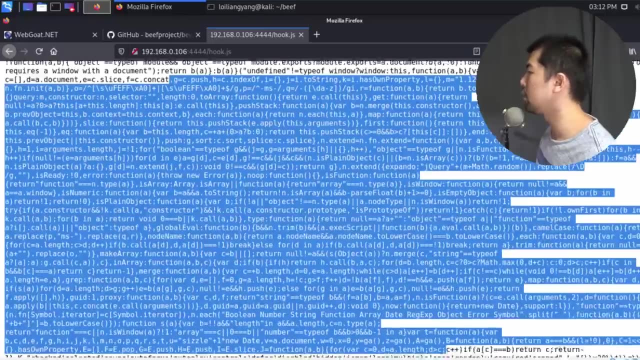 and I can click under the copy link address. I can go back to any browser and paste it over here and hit enter And this is all right. as you can see here, jQuery, JavaScript, all these different details right here- okay, and some parts of it. you can easily copy it and that would allow you. 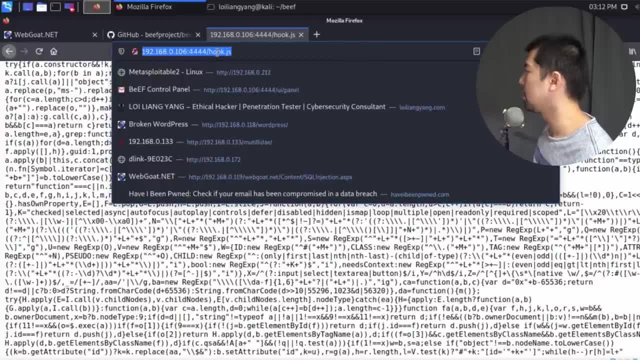 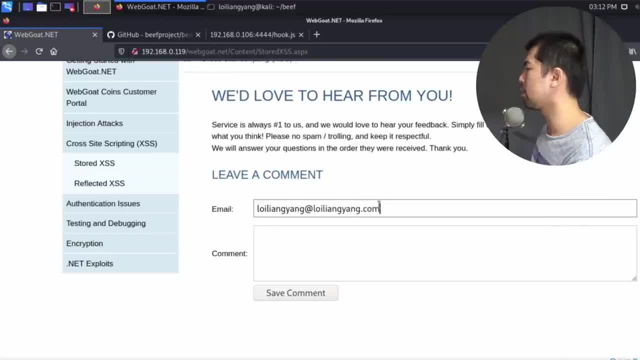 access to different components of a browser. So once you got a link, all right. all we got to do is ensure that we can copy the link, go back to the vulnerable website and in this case I can go and enter email. So I enter loyliangyang at loyliangyangcom and under the comment section, I can go and enter. 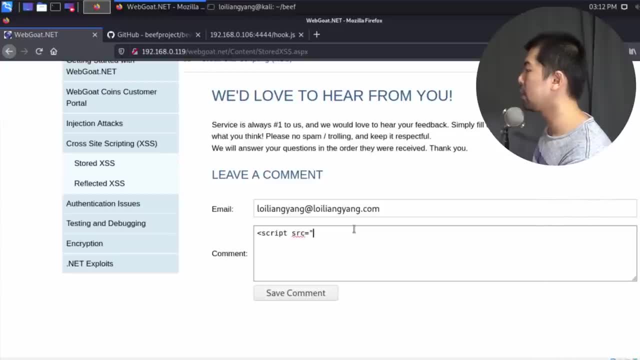 script source equal. okay, and I can do a double quote and paste the link which will point us to the JavaScript file, and I can now close the script. So once I close the script, I can go ahead and click save comment. All right, so here we go, We got it, We're in. We have just planted our malicious code. 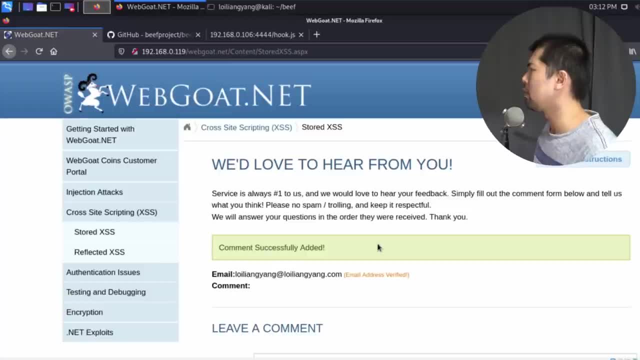 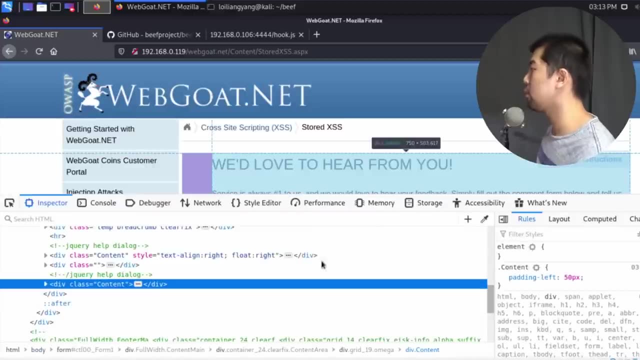 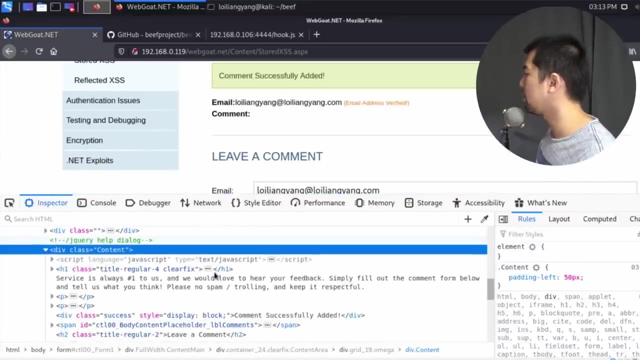 into the website, allowing us to track users and to control the entire website fully. So what we can do now is do a right click and click inspect element to see if our script got loaded. All right, so I can see here we have content, okay, as the following, and I can go ahead and open content and right here at the bottom left: 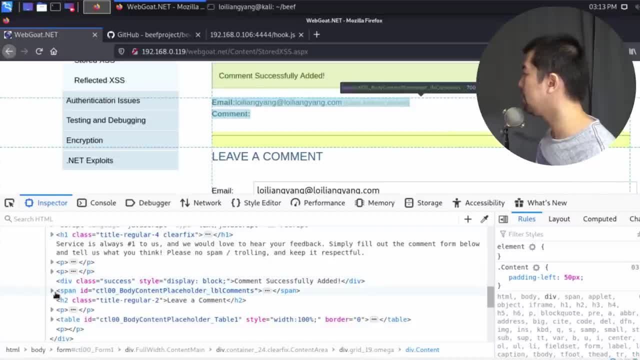 side, I can see the following: right, We have the email which is loyliangyang at loyliangyangcom, and right here we can see the following: all right, This is the part that we're looking for, So we have. 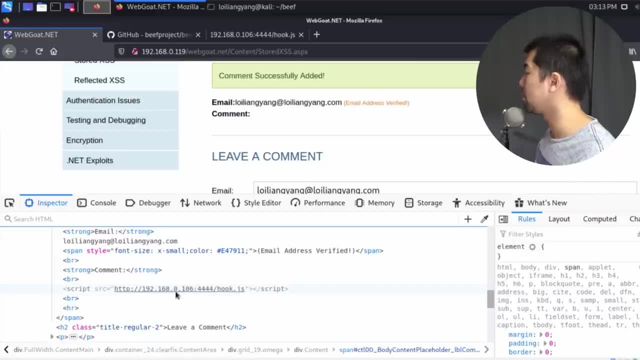 script source and we got 192.168.0.106,, which is our Kyle Linux machine, followed by the port number is 4444, followed by slash hookjs. All right, so we have planted our script into this site, which has a vulnerable comment section, and again, you can plant this anywhere. It can be a. 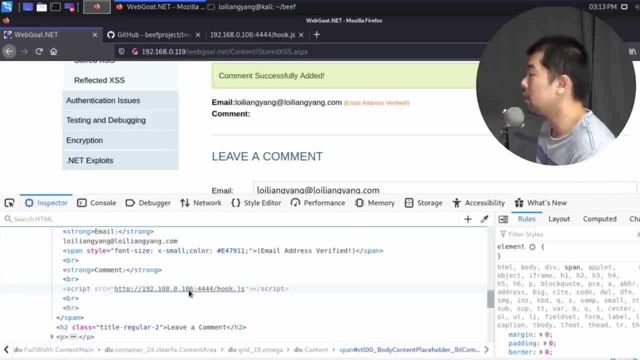 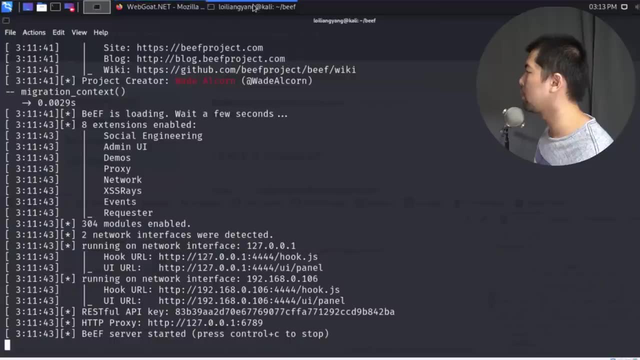 comment section, it can be on a review section, it can even be on a search section, and so on. So once you have it running, all we got to do next is to log in to browser exploitation framework. So, going back to terminal, all right, we have the link to the user interface. So all I got to do now. 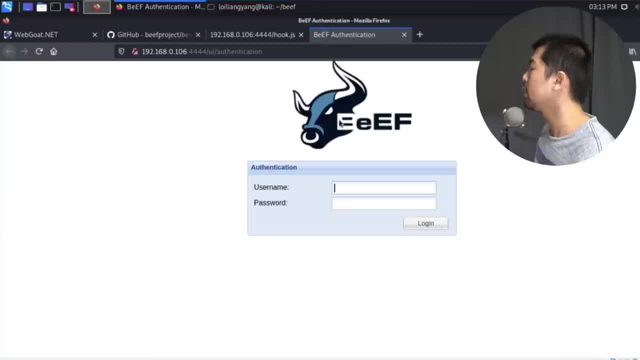 is right click on the UI panel, click open link and this will open up a new tab on Firefox or any browser. So go ahead and enter the username. So in my case I have the username of loyliangyang. enter a password I have set during the creation of browser exploitation framework and once we 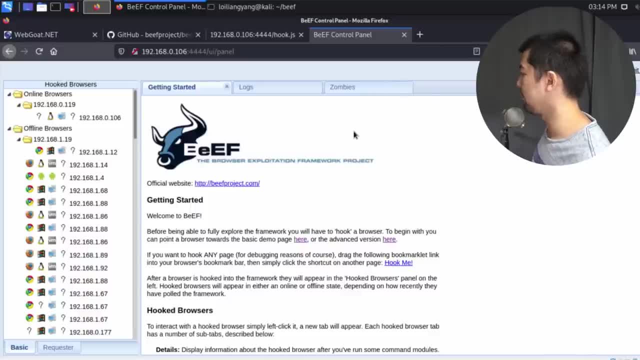 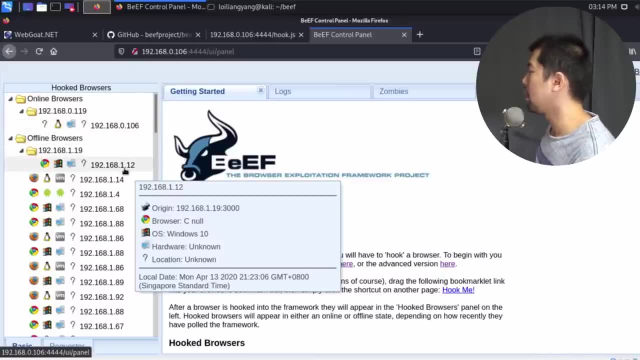 log in. you can see right here, All right on the left side, we have the following information. So let me zoom in a little more so that it is easier for you to see. So on the left side I have the IP addresses and I have the IP addresses of all those browsers who have came in and loaded the. 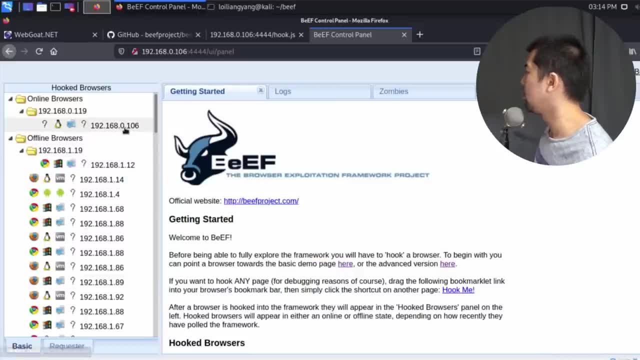 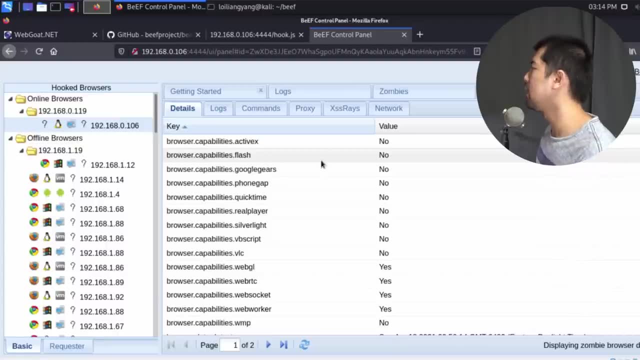 JavaScript that we have planted into any of these sites, And here we have the online browser. okay, So right here we can see that this is the browser that is currently inside the platform. And what to go back into another browser? okay, so this is my host browser that i'm doing all these tutorials. 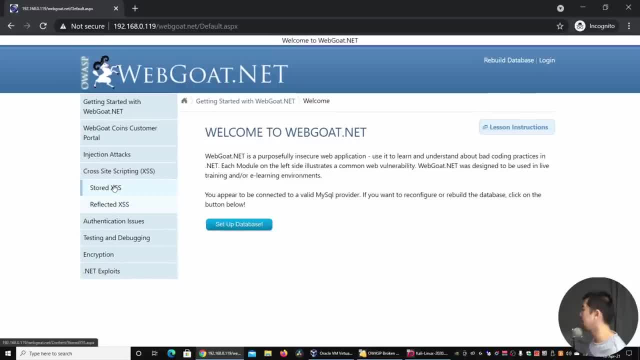 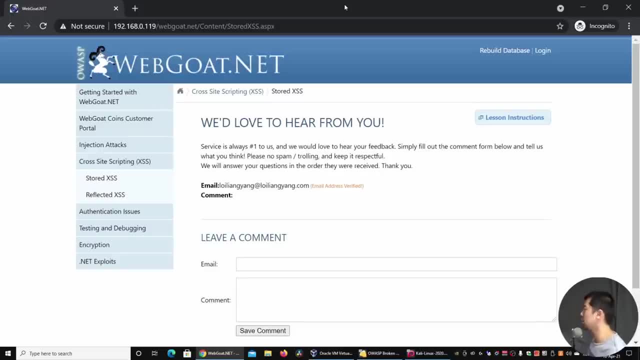 for you. and when i go under the cross-site scripting, i click on the stored xss and i clicked on it and what we are seeing here is that we have just loaded the script to, as you can see right here, email, as well as the comment section, which has the script, and we have verified that. 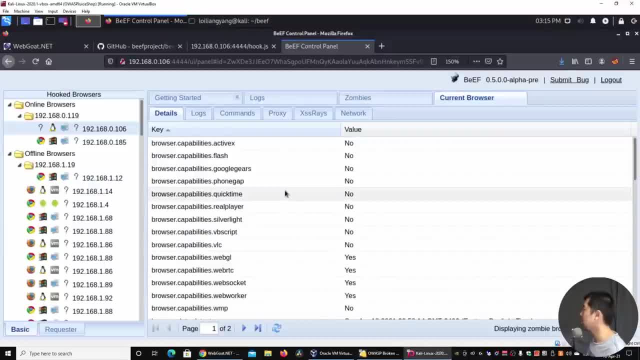 via inspect element. going back to colonics, we can see right here we have a new ip address coming in and we can tell that this is a windows 10 computer based on the pop-up that's showing right here on the left side, and we can see all the browser capabilities so that we can prepare. 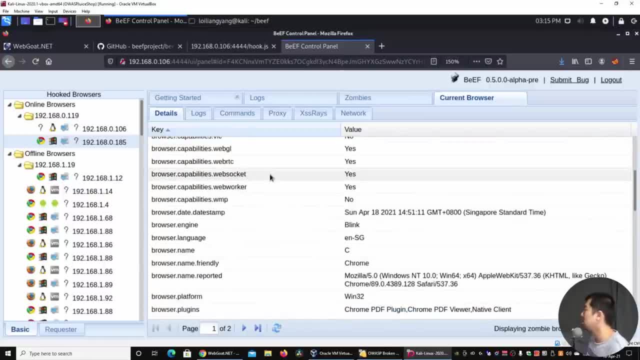 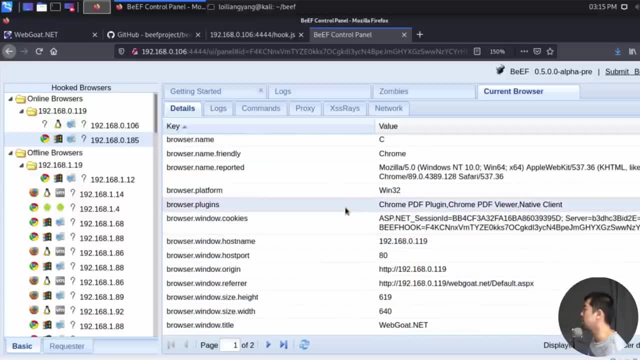 for the next type of cyber attack that we can launch against the browser. and, as you can see, here we have the date stamp, we have the browser language. so i am coming from singapore and we can see that there are certain plugins that a browser can take in. okay, so we can see all these details. 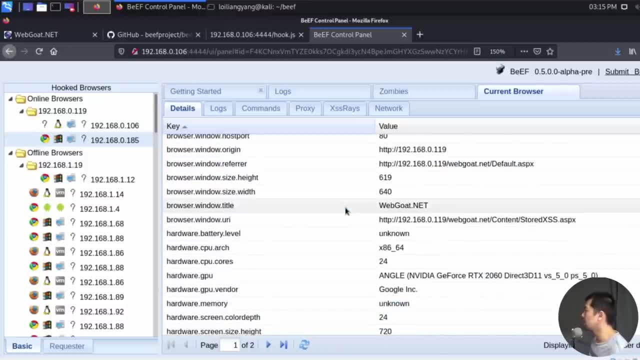 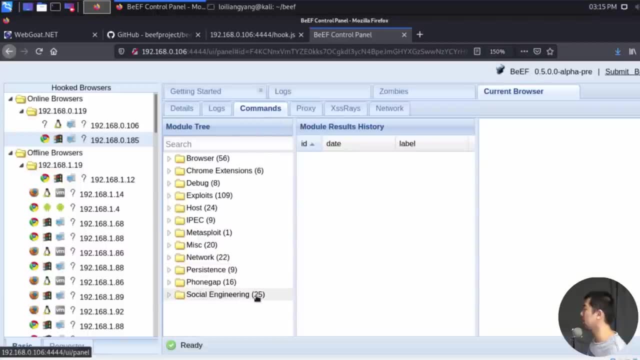 and all these different kind of data. but what's more interesting and more frightening is: what can we do now that we have loaded our code? what we can do is we can load our code and we can load the command in the command section and we can select under, say, for example, social engineering. 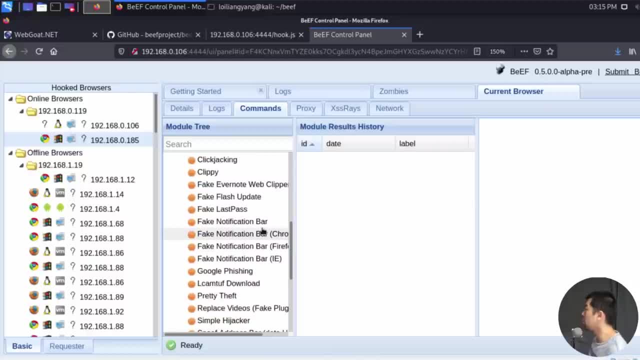 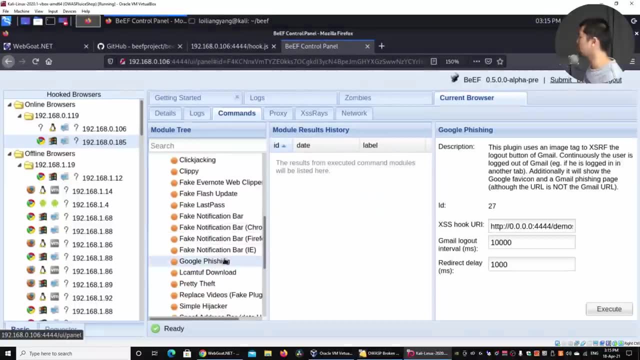 and right here. this is the part where we can actually control the website to display different kind of information back to the user. literally all i got to do is enter say, for example, google phishing, and i can click execute right. so once i click execute and what we can. 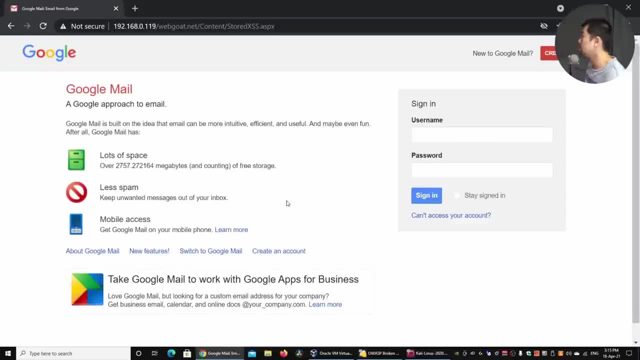 see next is when i go back to the browser, we are now being placed into a login page. and this is scary, isn't it? because all we did was go to an actual browser and we can see that we have a website. look at the comments. the next thing: you know you are hacked. what else can we do? going back, 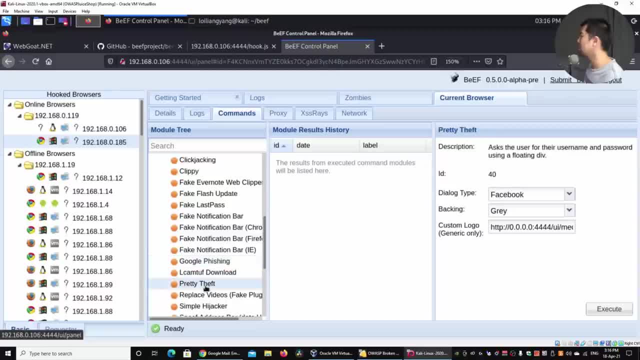 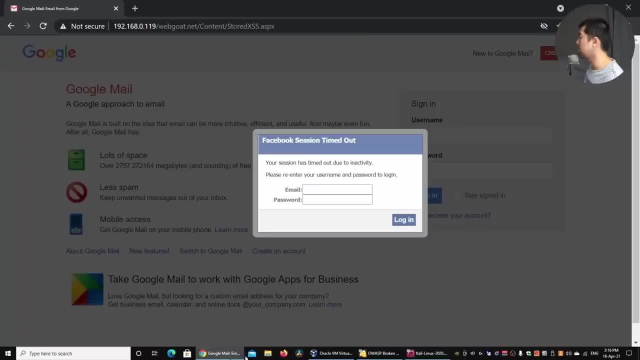 to colonics. going back to browser exploitation framework, i can select, say, for example, pretty tough, and again i'll now go ahead and click under execute. and going back to the browser, we see that there's a pop-up: facebook session time now. so very quickly there's a fake pop-up and say the user go.